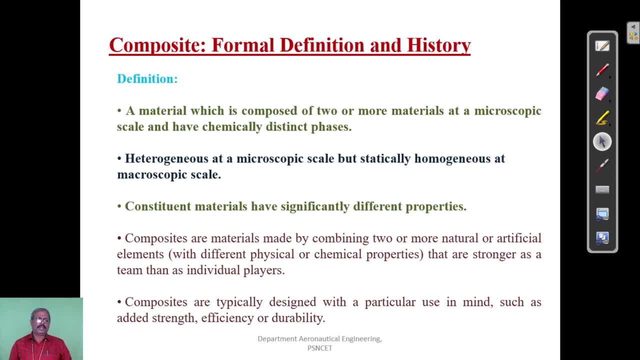 and have chemically distinct phases. The compositive materials are heterogeneous at a microscopic scale, but statically homogeneous at macroscopic scale. In composite material, the constituent materials have significantly different properties. Composites are materials made up of combining two or more natural or artificial elements. 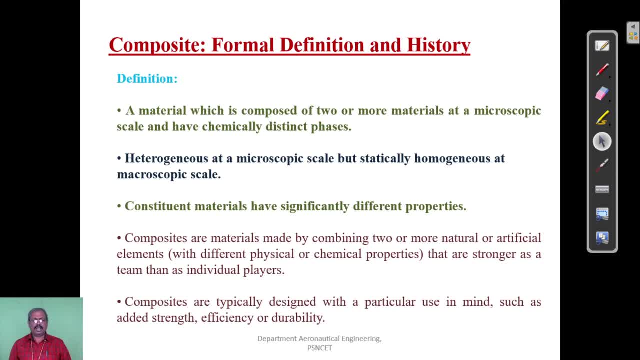 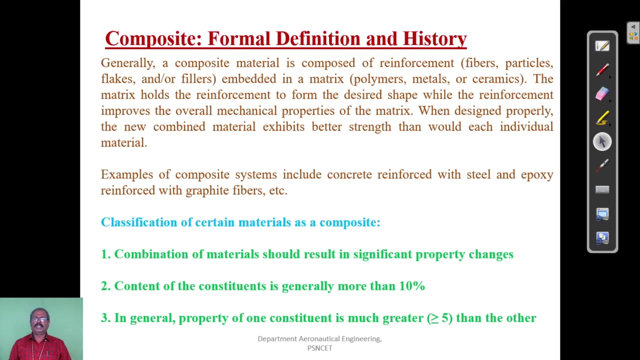 which are having different physical or chemical properties that are stronger as a team. Composites are typically designed with a particular use in mind, such as added strength, efficiency or durability. Generally, a composite material is composed of reinforcement ie, fibers, particles, flakes. 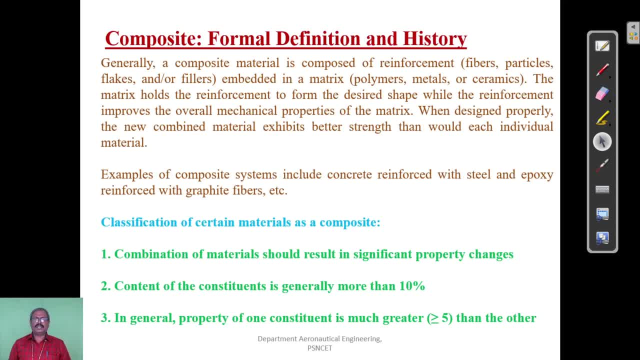 or fillers embedded in a matrix, like polymers, metals or ceramics. The matrix holds the reinforcement to form the desired shape, while the reinforcement improves the overall mechanical properties of the matrix. When designed properly, the new combined material expects better strength than would each individual. 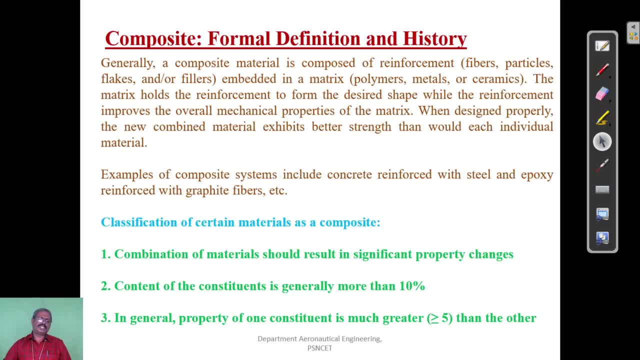 material. The examples of composite systems include concrete reinforced with steel. In the case of concrete reinforced with steel, the material is reinforced with steel. The material is reinforced with steel In case of RCC reinforced with steel. In RCC reinforced with steel, The steel rods are reinforced with concrete. 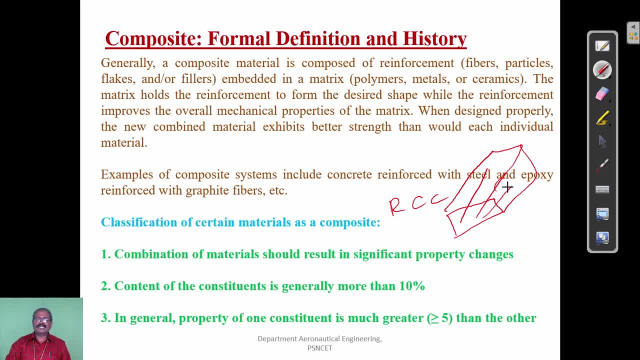 The concrete is a mixture of gravel sand, semen. This is called a matrix. This is an act as a matrix. in this RCC The steel rods are act as fibers reinforcement. So this is a best example for concrete reinforced with a steel. 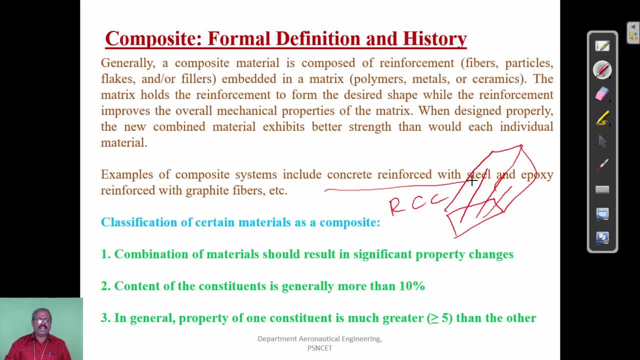 with a steel and epoxy reinforced with graphite fibres, etc. The classification of certain materials as a composite combination of materials should result in significant property changes. The content of the constituents is generally more than 10%. In general, property of one constituent is much greater than the other. 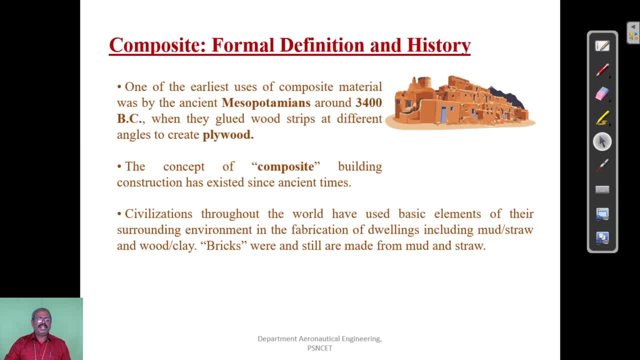 Come to the side of the history of composite material. One of the earliest uses of composite material was by the ancient Mesopotamians around 3400 BC, When they glue wood strips at different places, At different angles, to create plywoods Now we are calling plywoods. in 3400 BC, the Mesopotamians used these plywoods at the time. 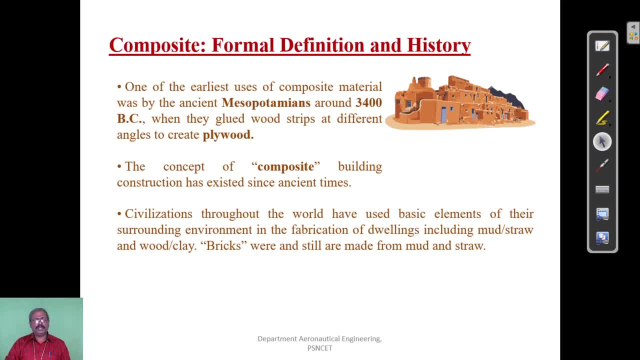 itself. The concept of composite building construction has existed since ancient times. Civilizations throughout the world have used basic elements of their surrounding environment in the fabrication of dullings, including mud or straw, and wood or clay Bricks were also used in the construction of the walls. 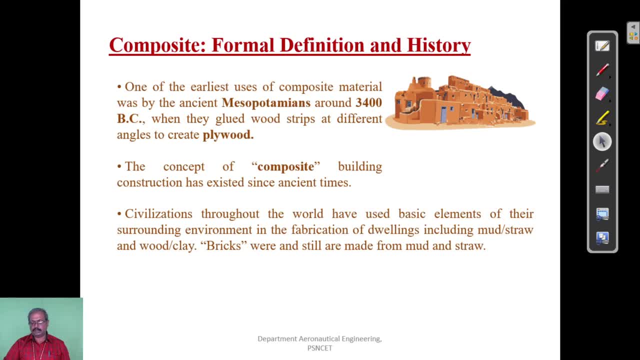 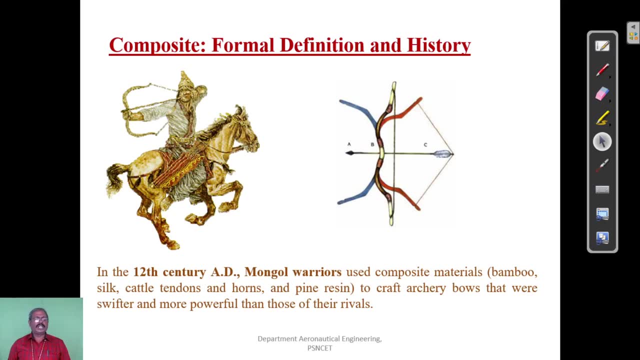 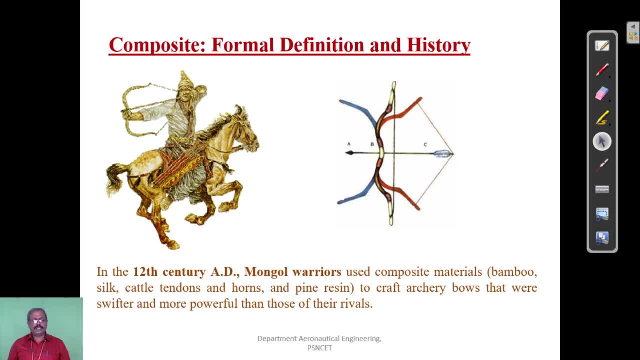 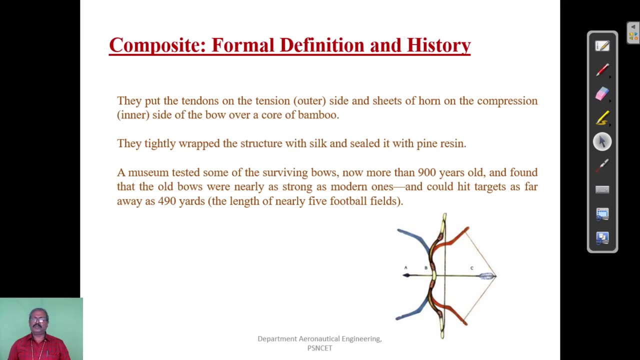 composed of bamboo, silk, cattle, dandans and corns and pine resin to craft archery bows that were sweeter and more powerful than those of their rebels. They put the dandans on the dendron. They put the dandron on the dendron side, that is, outer side of the bows and sheets of corn. 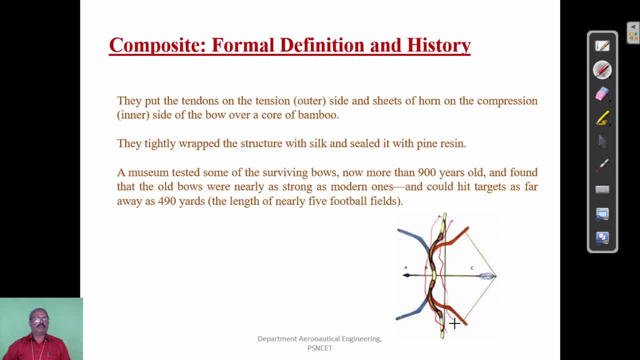 on the compression inner side of the bow over the core of bamboo. So bamboo is core. outer side they use the dandans and inner side they use sheet of corn. They tightly wrap the structure with silk and sealed with pine resin. So this is the composite. 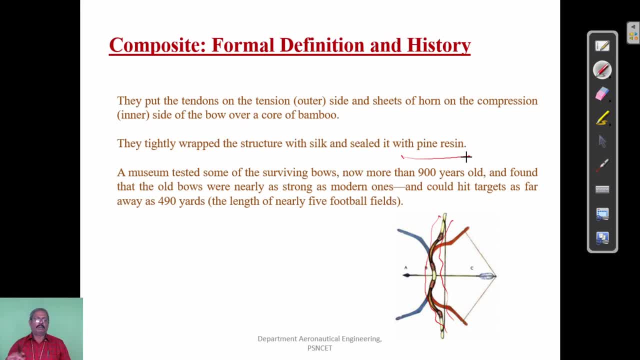 This is the composite material used for bow. A museum tested some of the surveying bows now more than 900 years old and found that the old arrows were nearly as strong as modern ones and could hit targets as far away as 490 yards, which is equal to the length of nearly 5 football fields. 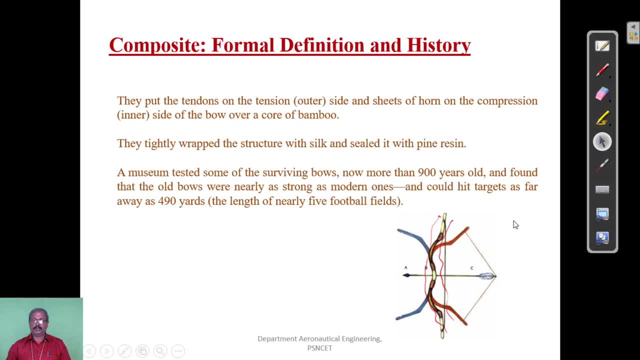 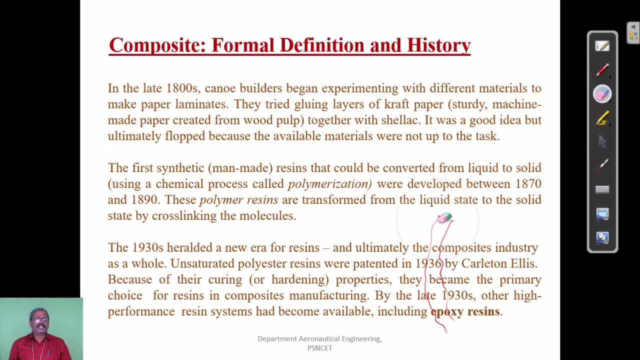 AVATAR. In the late 1800s, the Khmer builders began experimenting with different materials to make paper laminates. They tried blue layers of cracked paper together with shellac. It was a good idea, but ultimately flawed because the available materials were not up to the. 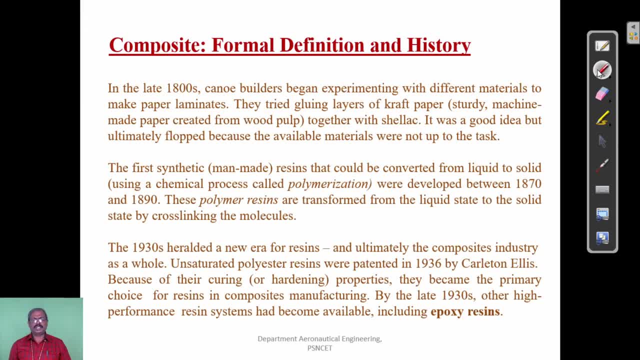 task. first, synthetic, that is, man-made. resins that could be converted from liquid to solid, which is the process called polymerization, were developed between 1870 and 1890.. These polymer resins are transformed from the liquid state to the solid state by cross. 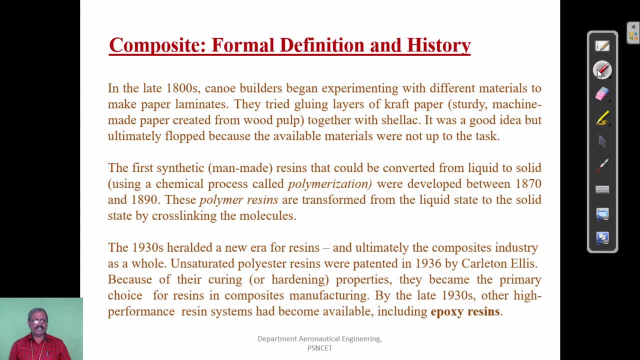 linking the molecules In 1930s heralded a new era for resins and ultimately the composite industry as a whole. Unsaturated polyester resins were patented in 1936 by Carlton Ellis. Because of their curing properties they become the primary choice for resins in composites. 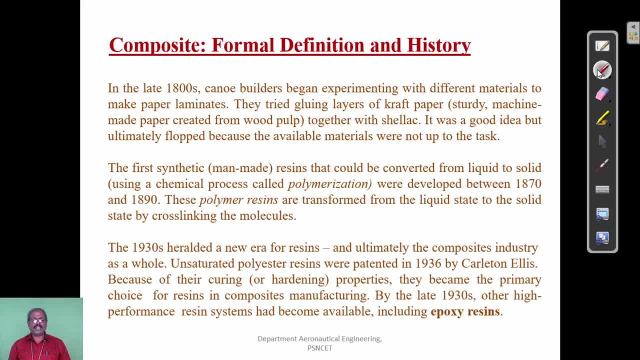 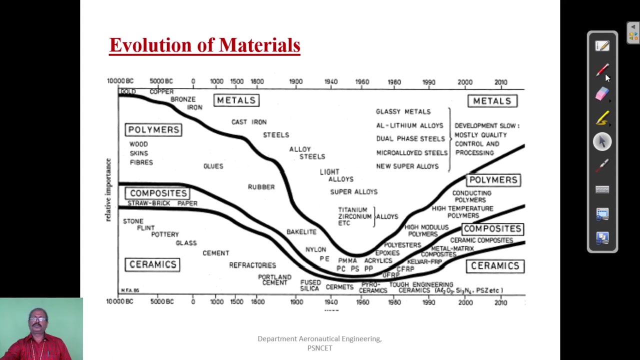 manufacturing By the late 1930s. other high-performance resin systems can become available, including abarxin These abarxin resins. nowadays itself, we are using this kind of abarxin resins in more composite materials. So this is the evolution of materials. 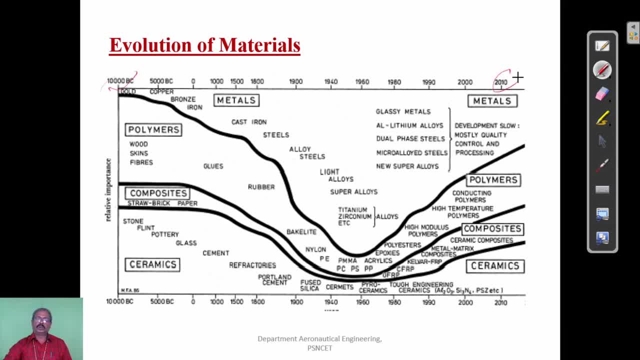 So it starts from 10,000 BC to now 2010 or 2020.. So metals, this is the relative importance of the materials. So in 1900 to 2000, we are giving more importance to metals but the composite in 10,000 BC itself. 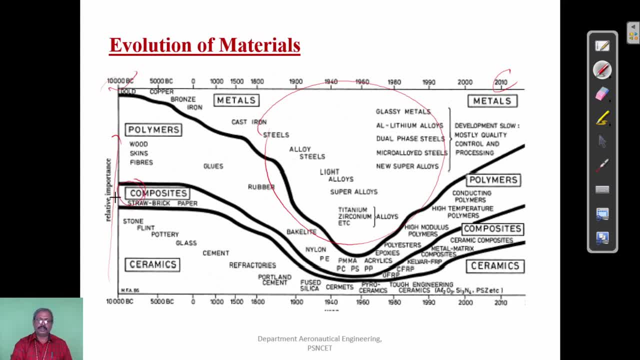 somewhat. they give the relative importance to composite materials. Nowadays the composites are used equivalent to metals, polymers and ceramics also. That is the overlap with the materials. When you see the composition of the material, then you think about the composition of materials. 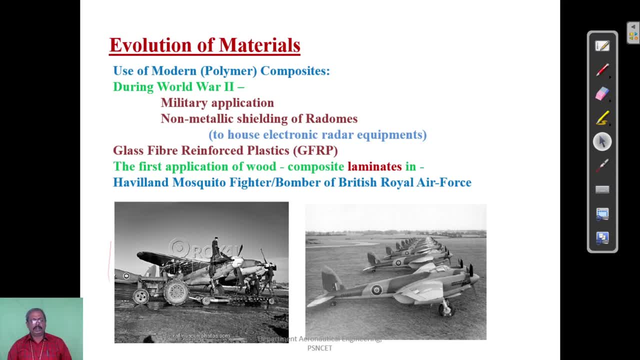 This is the information we are going to discuss in our next lecture. Reversible composite materials are used in the use of modern composites during the World War. In more military application they are using composite materials. particularly, they used the composite materials for non-metallic shielding of rodents to host electronic materials. 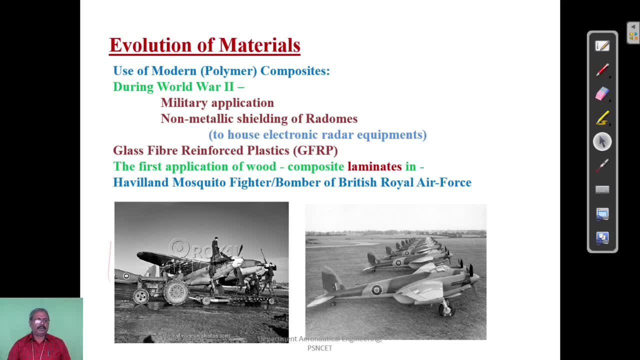 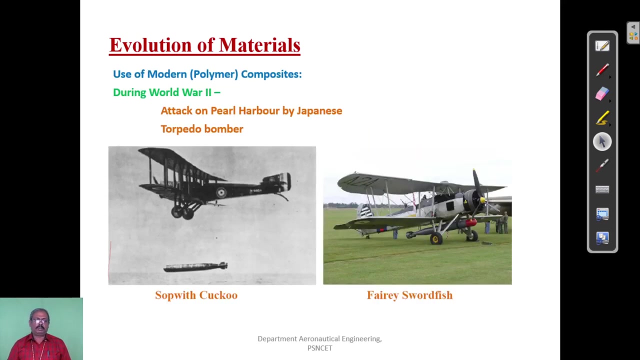 So that is the idea. The first application of wood composite laminates in Cavilland. Mosquito Fighter bomber of British Royal Air Force. During World War II in attack on Pearl Harbor by Japanese, the terminal bomber used. They used more of the parts, more parts in the terminal bomber, the composite materials. 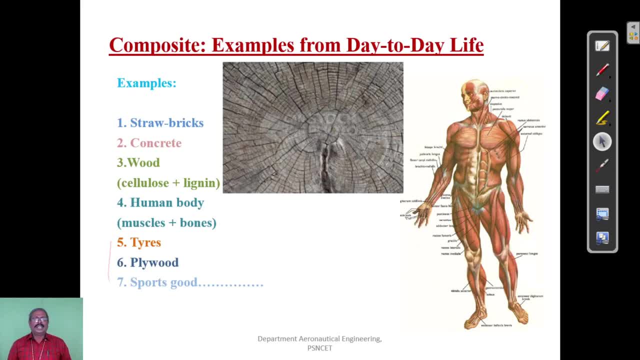 are used in that, The examples from day to day, like for the composite materials: straw bricks. one of the example for composite material: concrete. I already explained about this: concrete wood. this is combination of cellulose and lignin. Our human body itself is a composite material. 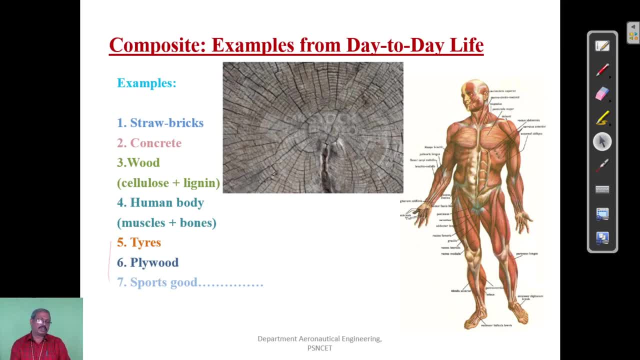 If we take a hand, bone is a reinforcement fiber and around the bone the muscles were surrounded to the bone and skin was upper side of the hand. So this is a composite material. Tyres in automobile industry: we are using the tyres. automobiles: we are using tyres. 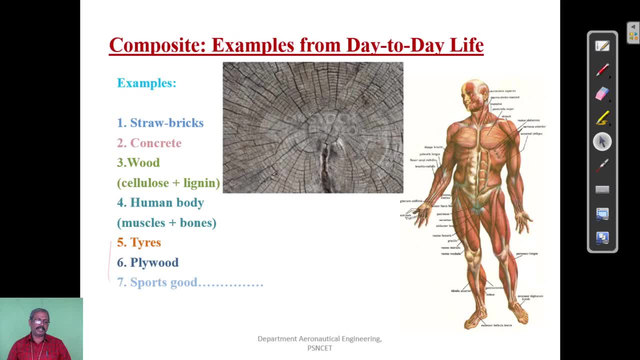 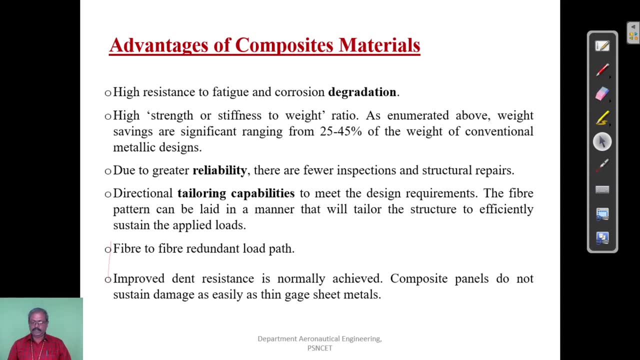 This is one best example for composite material. Ok, So the first application of composite materials: fly woods and several sports goods are made up from composite material. Then we come to the advantages of composite material. Composite materials have high resistance to fitting and corrosion degradation. 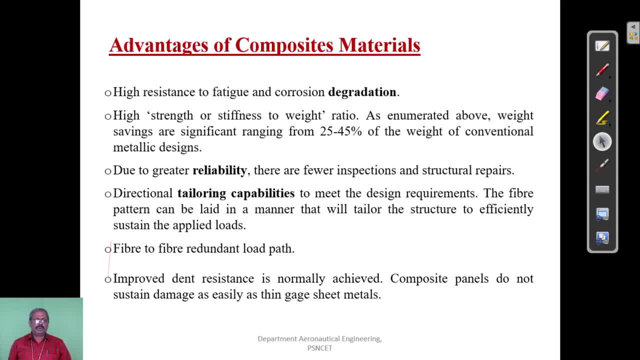 They have high strength to stiffness to weight ratio. strength or stiffness to weight ratio. As elaborated above. weight savings are significant ranges. ranges are determined ranging from 25 to 45% of the weight of conventional metallic design. Due to greater reliability, there are fewer inspection and structural repairs needed. 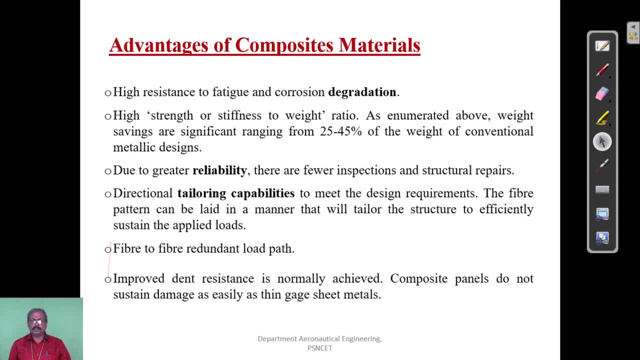 Directional dilating capabilities of the composite materials to meet the design requirements. The fiber pattern can be layered in a manner that will tailor the structure to efficiently sustain the applied loads. Due to fiber redundant load path, improved dent resistance is normally achieved in composite. 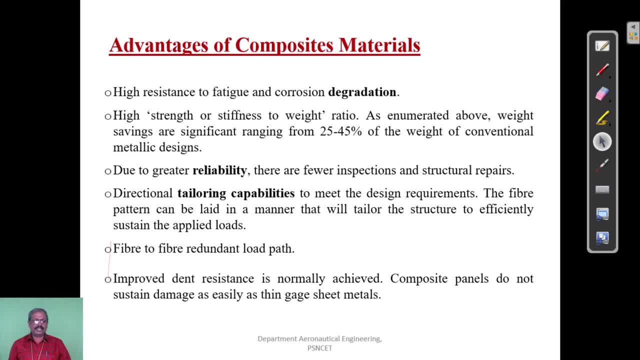 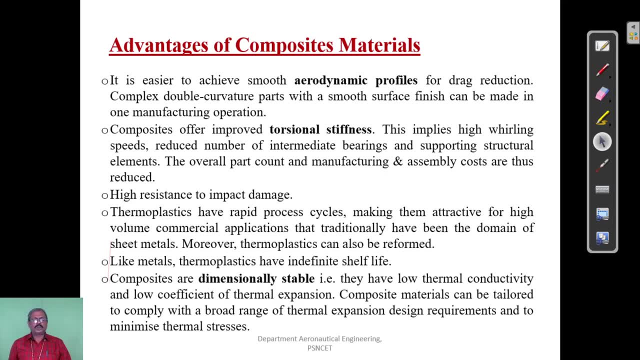 materials. So the composite panels do not sustain damage as easily as thin-gauge sheet metals. It is easier to achieve smooth aerodynamic profile for drag reduction in composite materials. Complex double curvature parts with a smooth surface finish can be made in one manufacturing. 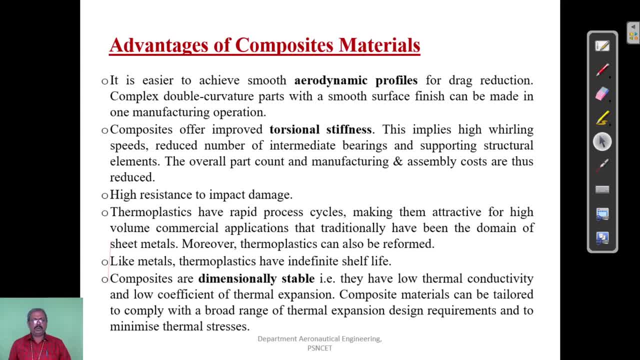 operation. Composite panels are made of a single material. Composites offer improved torsional stiffness. This implies high curling speed. reduced number of intermediate bearings and supporting structural elements. The overall part count in, and manufacturing and assembly cost are thus reduced. High resistance to impact damage. 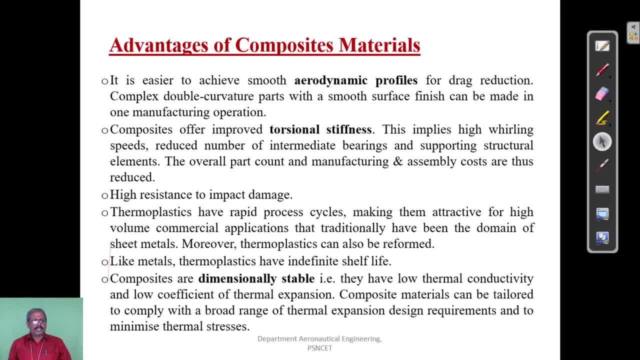 The thermoplastics have rapid process cycles, making them attractive for high body weight. Composite panels are made of a single material. Composite panels are made of a single material. Composite panels are made of a single material. Composite panels are very próximattly. 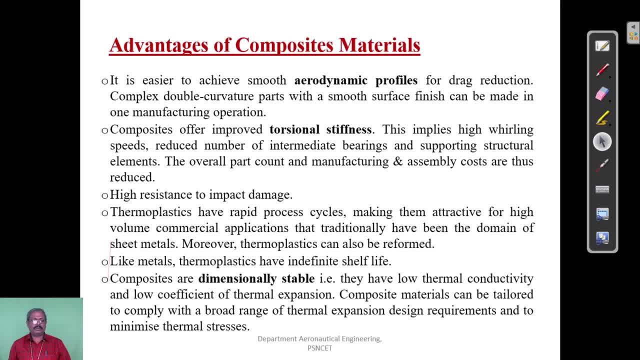 But low� in pressureial Luo and high tension. in modern mechanical equipment, TheALLais ideal effect is that the material is transparent\'a0our, especially coming to our California是這樣 applications that traditionally have been the domain of sheet. 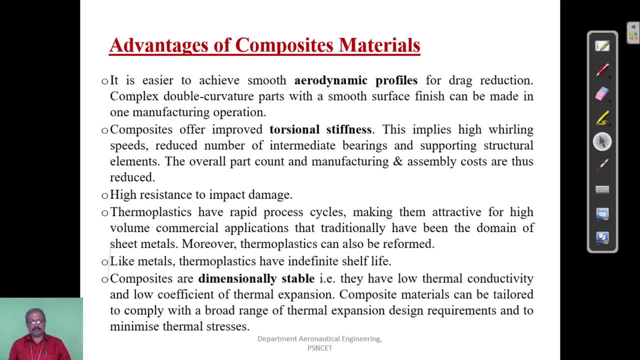 metals. Moreover, thermal plastics can be reformed Like metals. the composites In thermopl plastics have independent self. like Темoplastics have independent self. like Composite are diametrically stable, that is, they have low thermal conductivity and coefficient of thermal expansion. 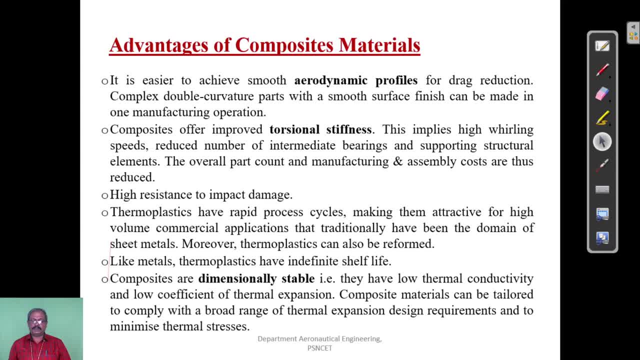 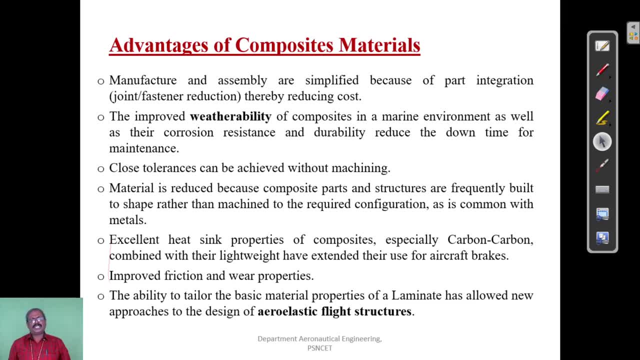 Composite material can be tailored to comply with a broad range of thermal expansion. What all how is the material consistent? It will be very good to use, to allowing design requirements and to minimize thermal stresses. Manufacturing and assembly of composite materials are simplified because of part integration. 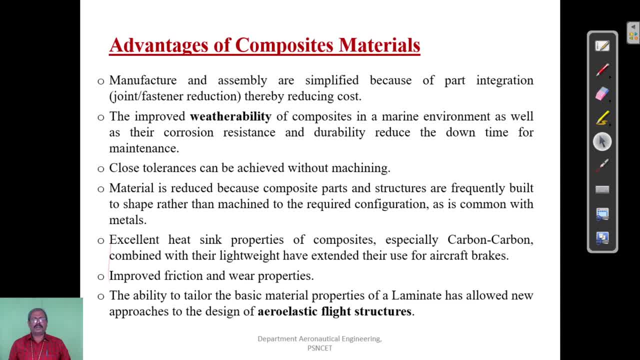 thereby reducing cost. The improved weatherability of composites in a marine environment, as well as their corrosion resistance and durability, reduce the down time for maintenance. Close tolerance can be achieved without mentioning in composite materials. The material is reduced because composite parts and band structures are frequently built. 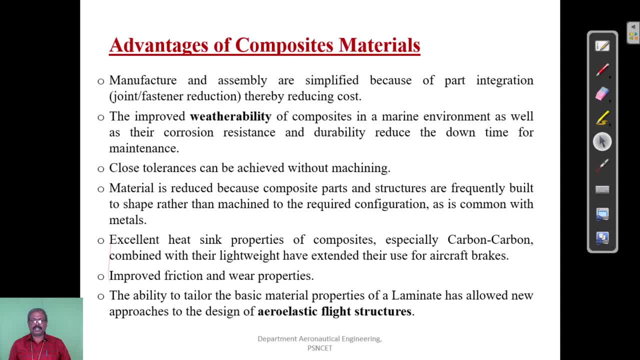 to shape rather than machined to the required configuration, as is common with metals. Excellent heat sink properties of composites, especially carbon-carbon, combined with their lightweight, have extended their use for aircraft brakes. Composite materials have improved friction and wear properties. The ability to tailor the basic material properties of a laminate has allowed new approaches to 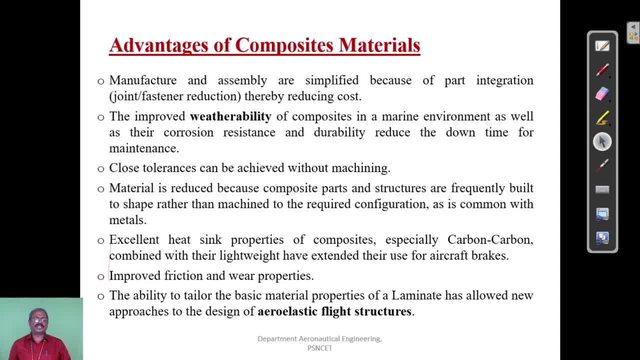 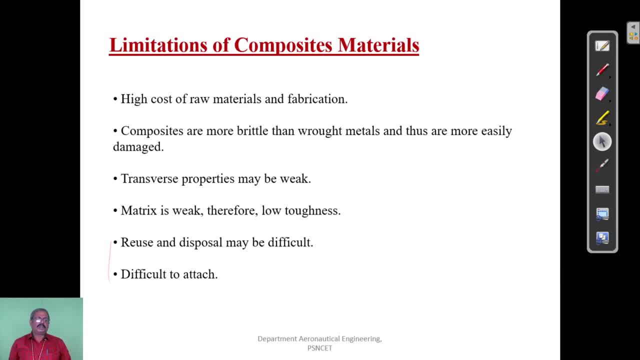 the design of aero-elastic flight structures. Some of the limitations of composite materials are high cost of raw materials and fabrication. Composites are more brittle than rock metals and thus are more easily damaged. Traverse travel is a major problem. Composite materials are more fragile than rock metals and thus are more easily damaged. 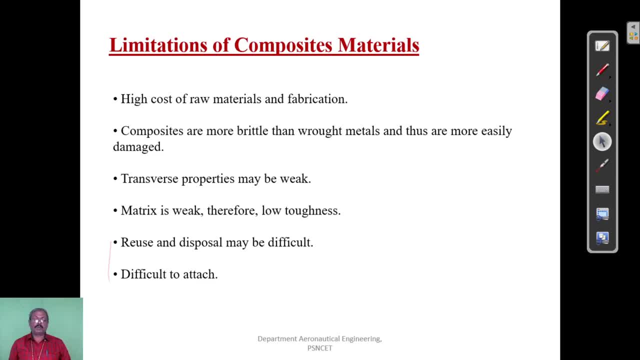 Traverse travel is a major problem. Composite materials are more fragile than rock metals and fabrication Transverse properties may be weak in composite materials If the matrix is weak, therefore, toughness is low. Pre-use and disposal of composite materials may be difficult. The composite material- parts made from composite materials, are difficult to attach with other. 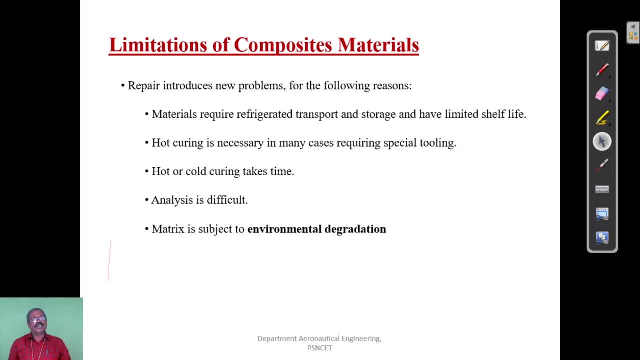 metal parts Repair introduced new problems for the following reasons: Materials require refrigerated transport and storage, height transport and storage and have limited shelf life. Hot curing is necessary in many cases, requiring special toolings. Hot or cold curing takes time somewhat, days or hours. 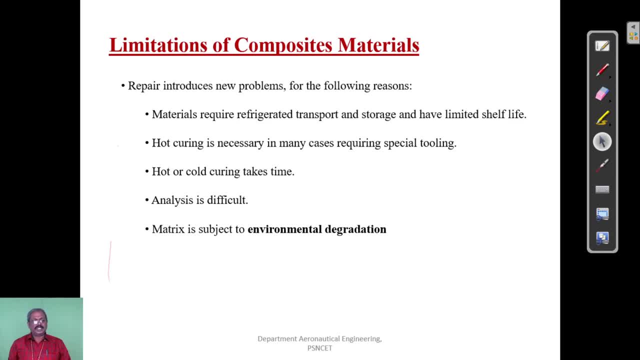 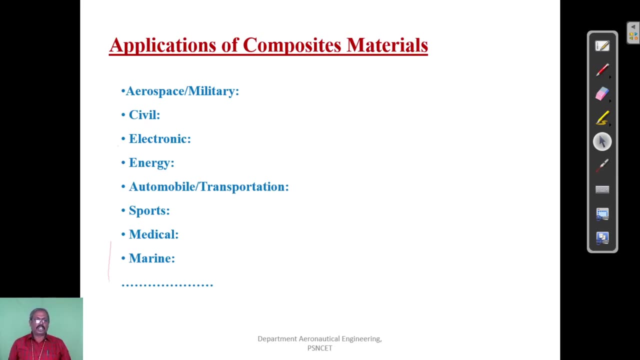 The composite material parts analysis is very difficult. Matrix is subject to environmental degradation. So these are the limitations of composite materials. Now the application of composite materials in various fields: aerospace or militaries, civil electronic applications, energy application, automobile transportation, sports, medical. 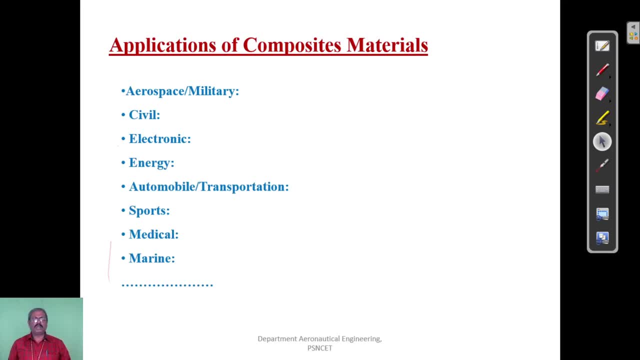 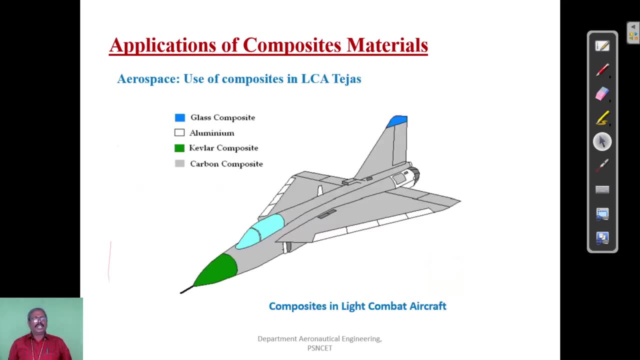 marine, etc. So these are the fields, almost all the fields- we are using composite materials nowadays. So in aerospace, the use of composites in various fields We are using glass composites in LCA, Tejas, glass composites. here you are using glass. 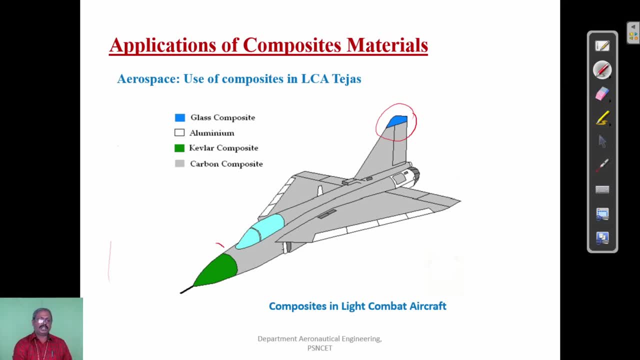 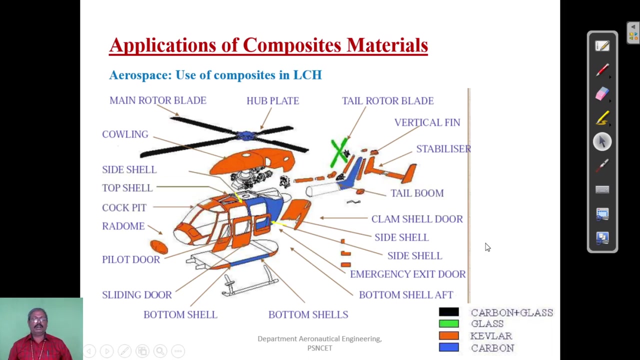 composites in tail parts: ok. Kilvore composite in nose of LCA Teja. carbon composite in body: ok. So these are the composite materials used in parts in the LCA Tejas. This is the dismantled view of helicopter LCH. 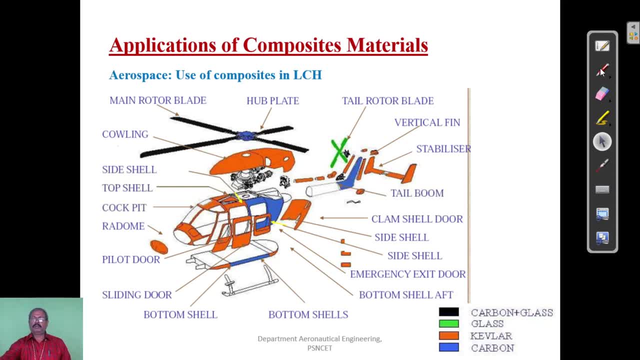 So here we are using so many parts made up of composite materials like carbon glass material, carbon glass material, glass composites, Kelvin composite for body parts and carbon composites in several parts. okay, This is another example of composite materials used in aerospace industries. 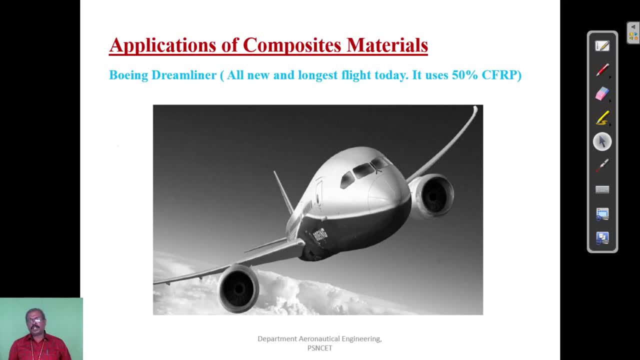 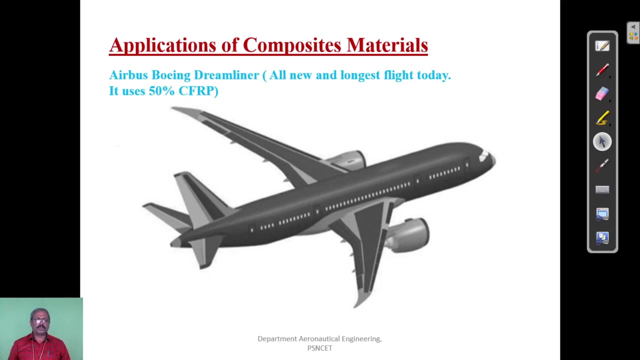 Boeing Dreamliner is an all new and largest flight today. It uses 50% of carbon fiber reinforced polymers. CFRP means Carbon Fiber Reinforced Polymers. the same flight, the Airbus Boeing Dreamliner. They are using carbon fiber reinforced polymers in 50% of its parts. 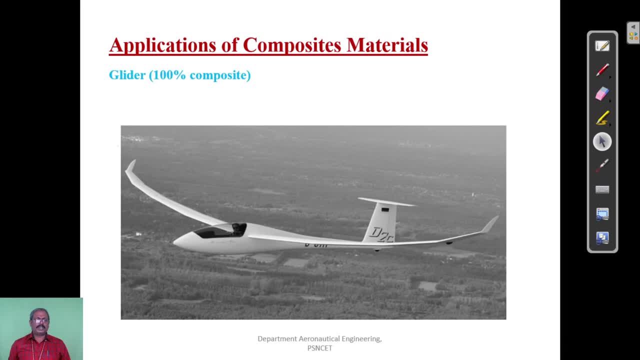 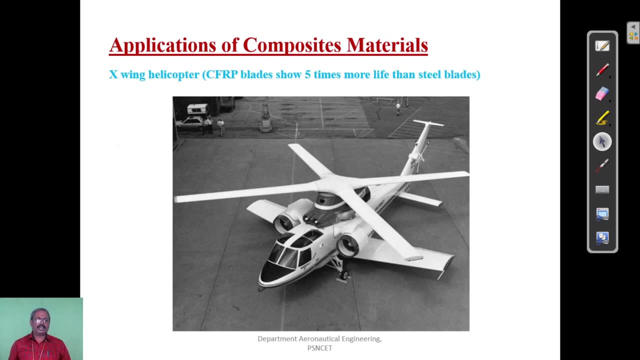 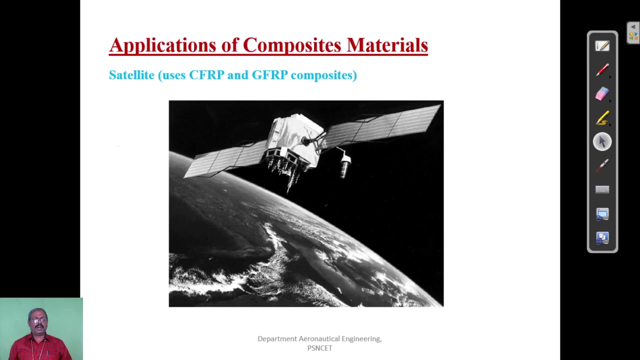 This is a glider. 100% of composite materials used in all the parts in this glider. This is a X-Wing helicopter. the carbon fiber reinforced polymer blades shows five times more light than steel blades. In satellites we are using so many parts. 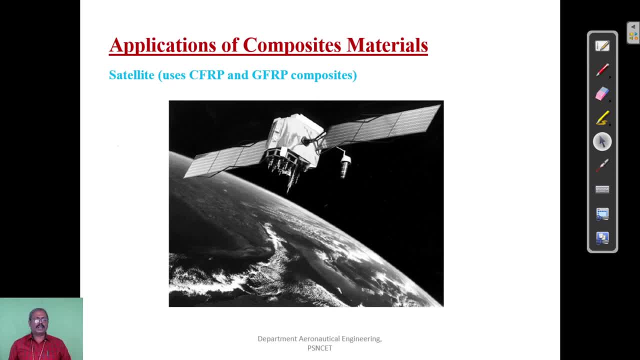 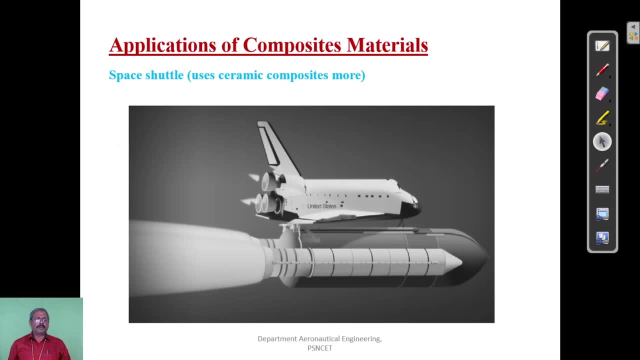 Made up of CFRP, that is, Carbon Fiber Reinforced Polymer and Glass Fiber Reinforced Polymer composites In space shuttles. the ceramic composites are used in various parts because of the heat applications. This is a cross-sectional view of a composite blade. 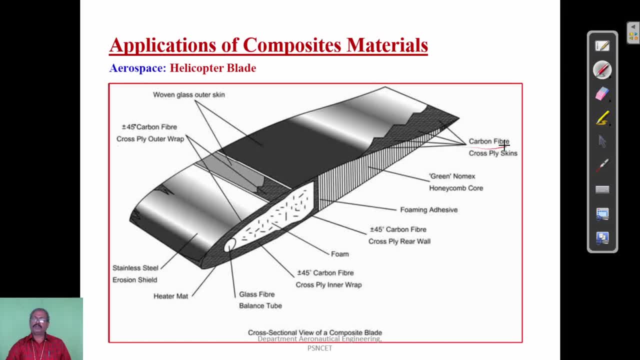 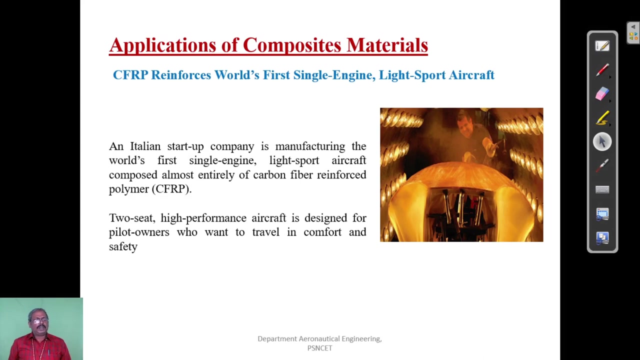 In this blade. they use carbon fiber, green carbon fiber, carbon fiber, carbon fiber green, NOMACS, honeycomb ore, carbon fibers, glass fiber- so many composite materials used in this helicopter blade. Carbon fiber- reinforced polymer reinforces Wells's first single-engine light sport. 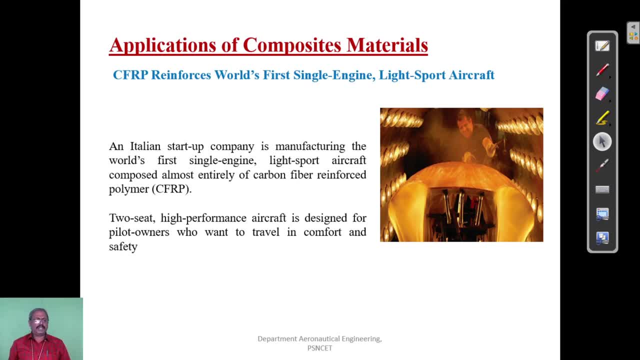 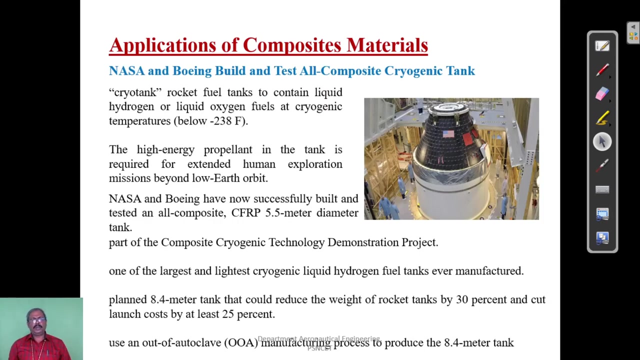 aircraft. An Italian startup company is manufacturing the Wells's first single-engine light sport aircraft, composed almost entirely of carbon fiber reinforced polymer. This two-seater high-performance aircraft is designed for pilot owners who want to travel in comfort and safety. NASA and Boeing build and test all composite cryogenic tanks. 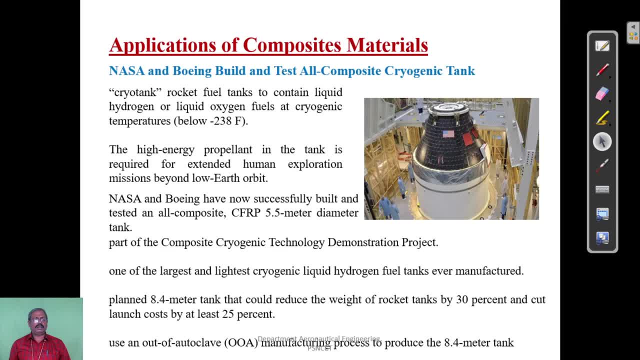 Cryo-tank rocket fuel tanks to contain liquid hydrogen or liquid oxygen fuels at cryogenic temperatures. These fuel tanks are equipped with a high-energy propellant which is below minus 238-degree Fahrenheit. The high-energy propellant in the tank is required for extended human exploration missions beyond. 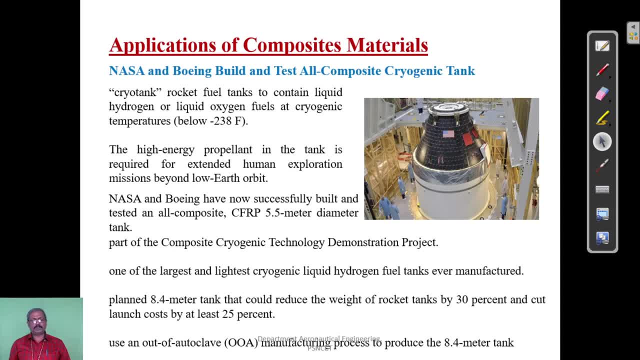 low Earth orbit. NASA and Boeing have now successfully built and tested an all-composite CFRP 5.5-meter diameter tank, part of the Composite Cryogenic Technology Domestic Project, one of the largest and lightest cryogenic liquid hydrogens. The plant's 8.4-meter tank could reduce the weight of rocket tanks by 30 percent and 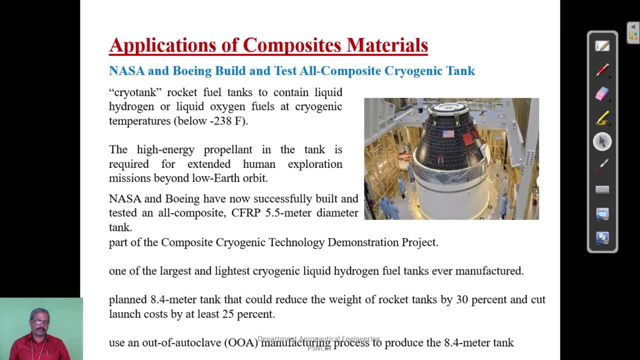 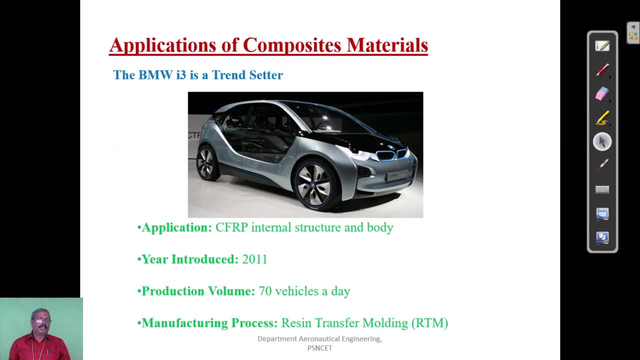 cut launch costs by at least 25 percent. They use out-of-autoclave manufacturing processes to produce the 8.4-meter tank. automobile side, The BMW i304 is a large one. This is the current model. The Celebrate 작전lies have a large engine, but with its short engine it is US $1.08 per. 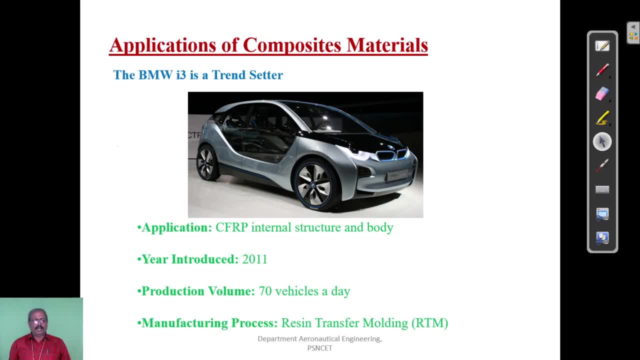 trendsetter car. It is a best example for application of carbon fibre reinforced polymer. They use the CFRP for internal structure and body of this BMW i3. They introduced this car in 2011.. The production volume of this car is 70 vehicles per day. The manufacturing 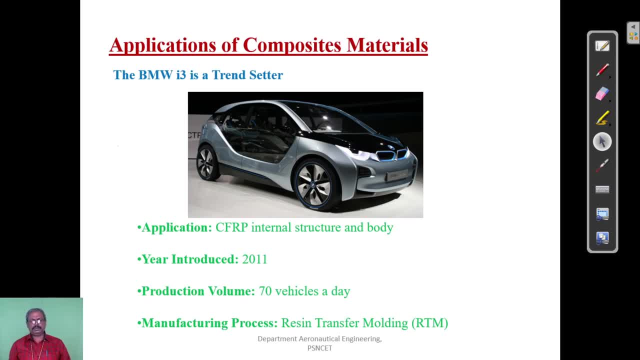 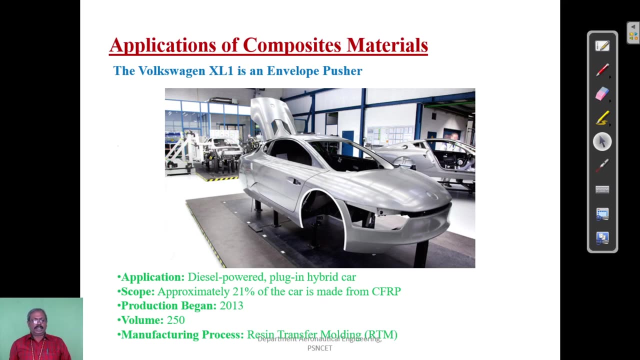 process to make the composite materials. RTM, that is, Resin Transfer Moulding, is what produces the composite parts. The holes were XL-1,, which is an application of composite materials. Approximately 24% of this car is made from CFRP. 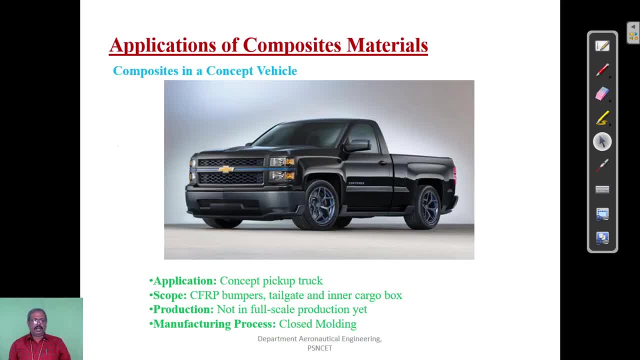 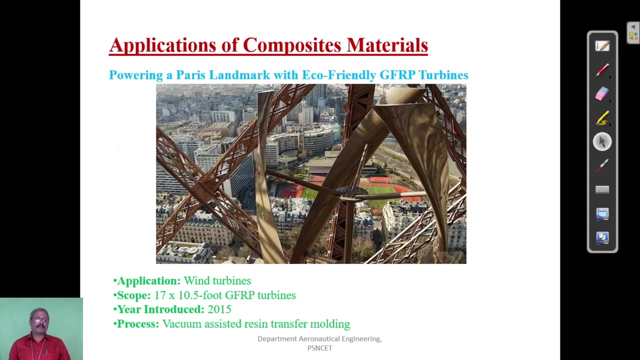 Then this is a Chevrolet concept vehicle. in this vehicle they use a composite for pumpers, they use carbon fiber reinforced polymers, tailgate and inner cargo box. Then application of composite materials in wind turbines powering a Paris landmark with that is E-field tower, with eco-friendly GFRP, that is glass fiber, reinforced polymers, turbines. 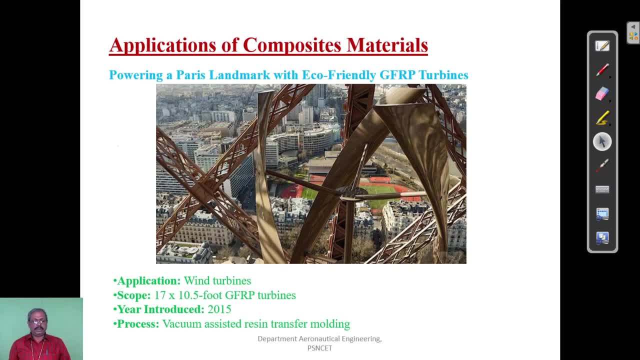 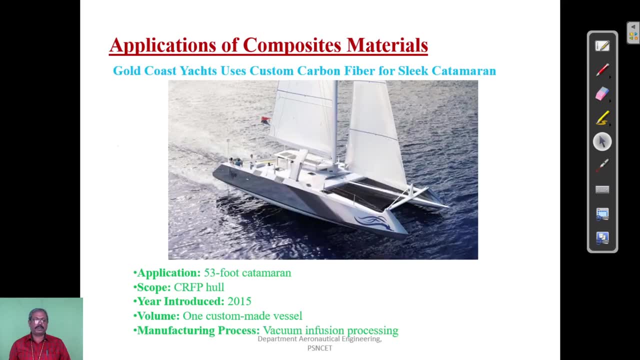 So this is a 7 into 10.5 feet GFRP turbines. it is introduced in the year of 2015.. They use the back foam acetate resin transfer molding to make this parts of this turbine. This is a Gold Coast Yatchis. 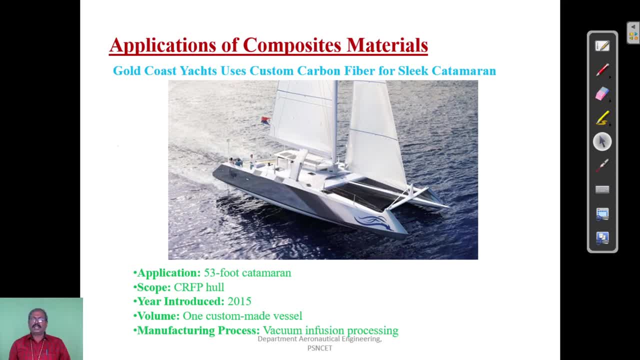 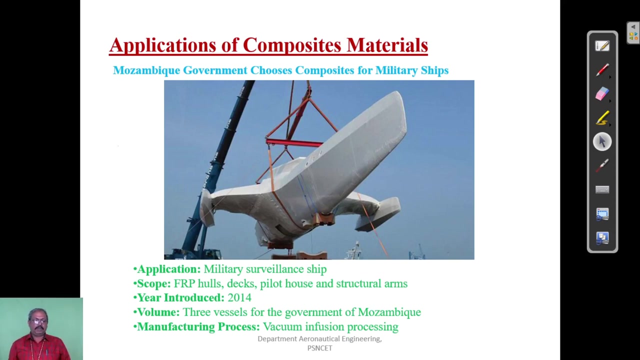 It uses custom carbon fiber for slick catamaran. They use composite materials to make hull of this catamaran in the year of 2015.. They use vacuum infusion processing to manufacture the hull. Then this is a military ship. They use a composite materials in this ship. 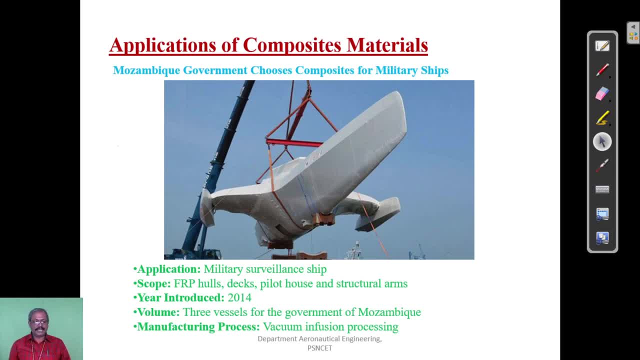 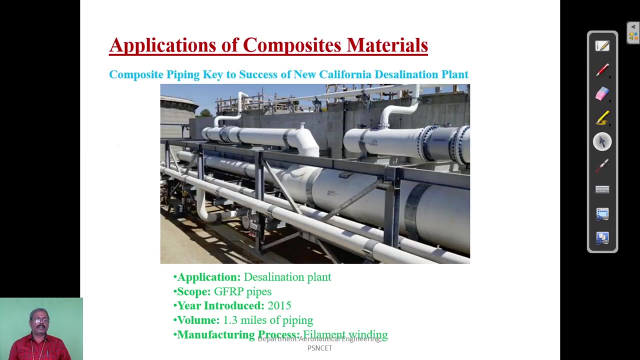 FRP- Fiber Beam Processing, Then this is a military ship. They use composite materials used to manufacture this sponge. These are truly rate of conversion materials from the N груys. So this is the number of passenger parts, different types of spare parts, different. 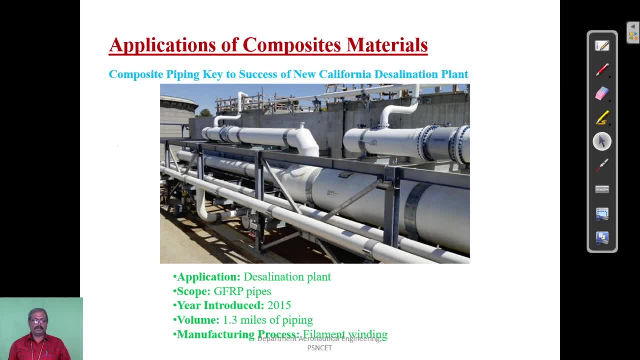 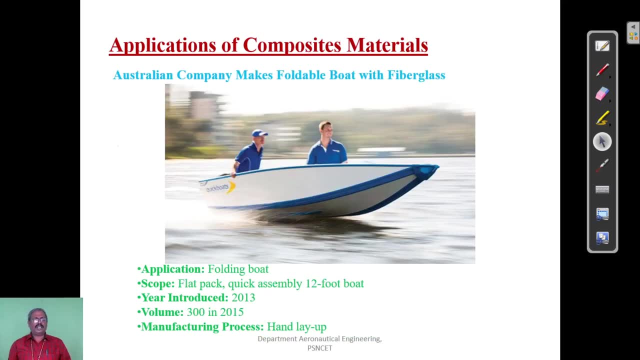 modules, different-structure. The wholeサ Guinness label of the plataforma is Gauss-Weiss. it is easily describe and being included in the design. Pop P yum GFRP pipes in this desalination plant. okay, this is an Australian company makes foldable.